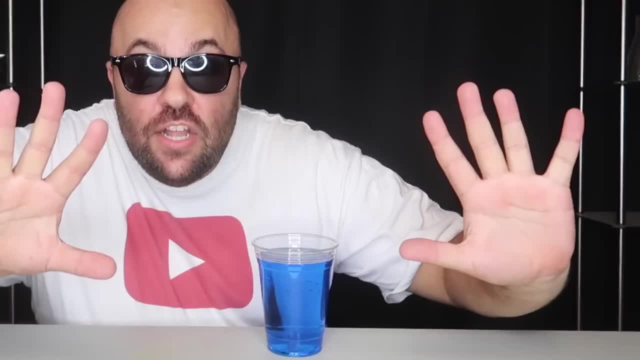 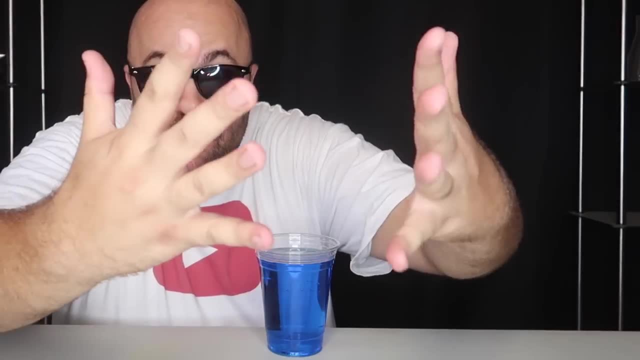 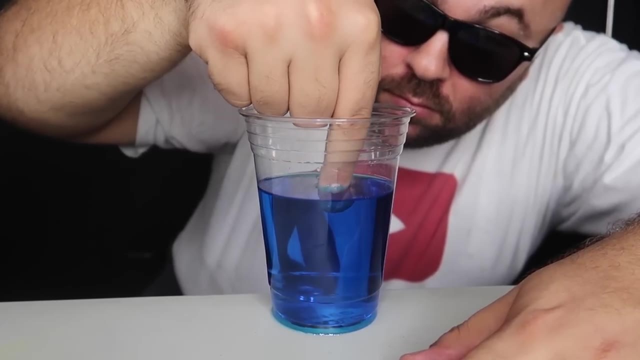 your finger is magically healed back onto your hand. Here's a really amazing hand trick that you can do Bare hands. right here and I have a cup of water on the table Watch. I take my finger just like this. I'm going to dip it in the water and look what happens: My finger actually drinks the. 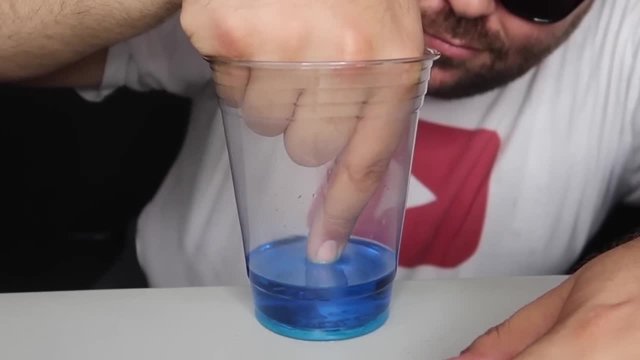 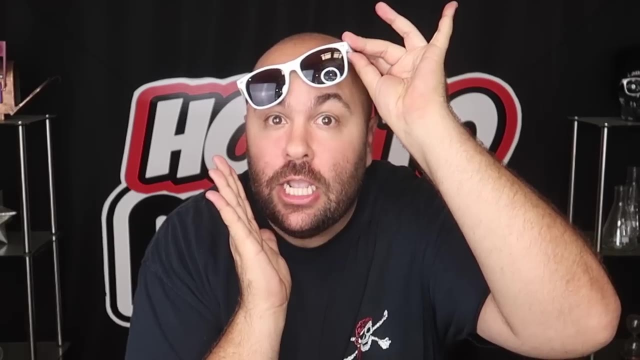 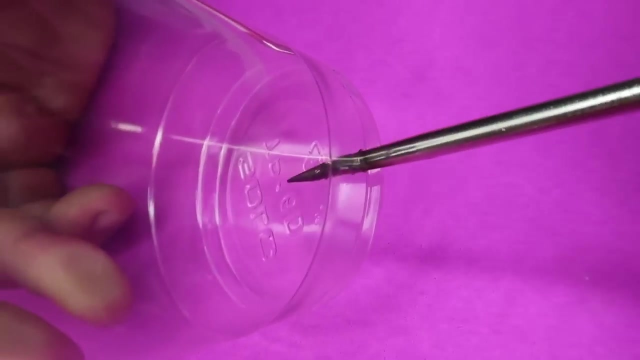 water from the cup. It was thirsty. All right, here's how it's done. I'm about to reveal a secret. The secret to this trick is extremely simple, and I'll teach you how it's done right now. Grab a plastic cup to set this up, and 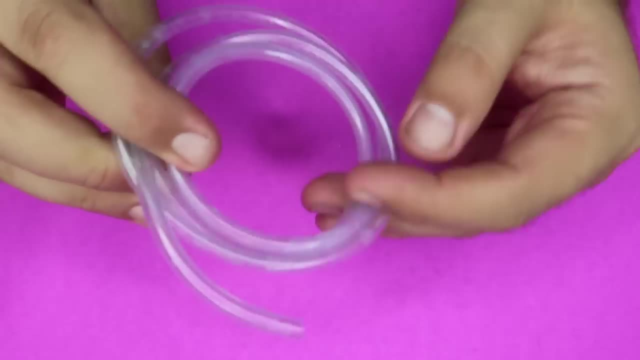 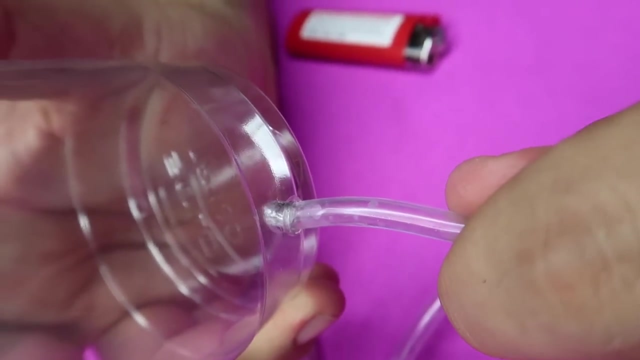 poke a hole in the bottom of the cup. You're also going to need a piece of plastic tubing like this is used for aquariums, fish tanks, stuff like that. Take the tube and plug it into the bottom of the cup, just like this. This is very similar to the boiling water trick that you saw in our last. 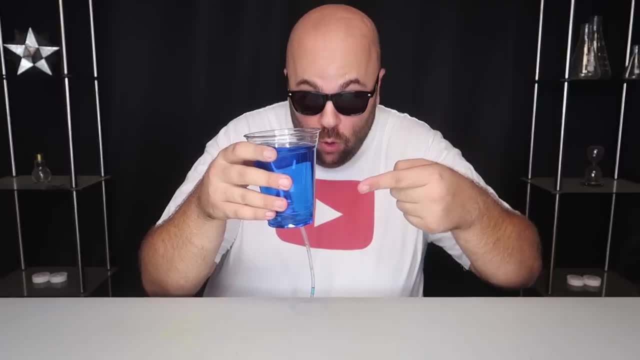 episode of How to Magic, Kind of the reverse of it. You're going to need a piece of plastic tubing like this: Once you have the cup filled with water, you're going to set it on the edge of a table, just like this, and let the tube drape across the back of the table, hidden below the table from. 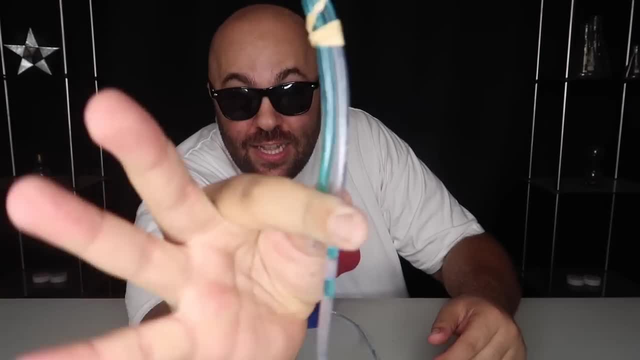 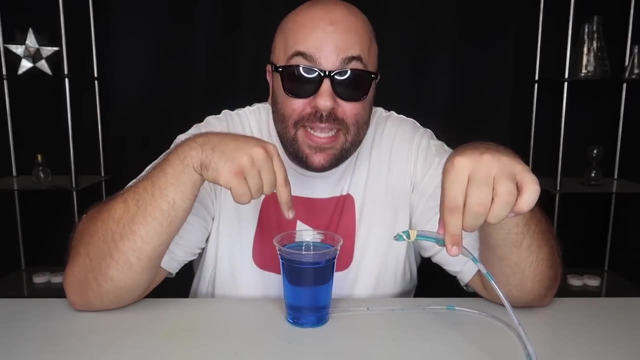 the audience's view. Also, add a rubber band to the end of the line so that the liquid does not leak out. You're going to have this below the table and have an assistant down there. remove the rubber band and open the line so that the liquid begins to drain from the cup. You can have another cup. 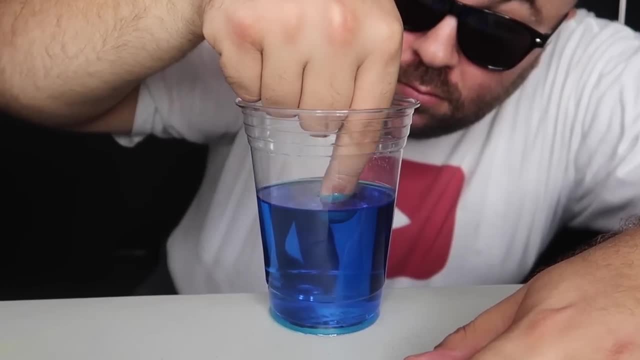 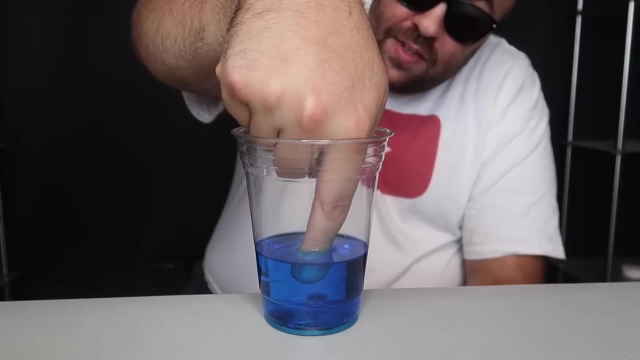 down there to drain the liquid into, and it looks like your finger is just magically drinking the liquid inside the cup. So as the water leaks out the tube into the cup, below that water is going to level sinks and it looks like your finger, your hand, is just somehow drinking the water. The 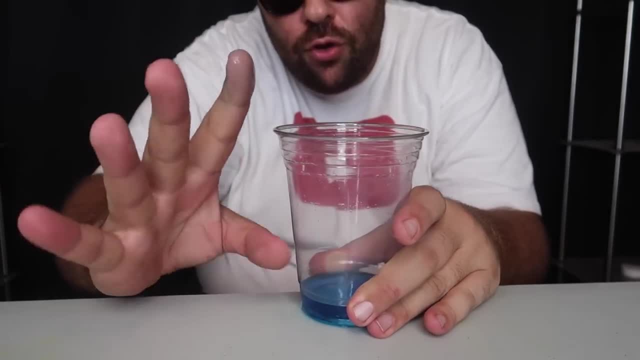 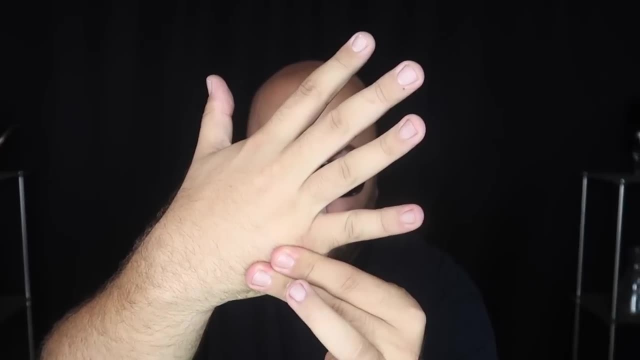 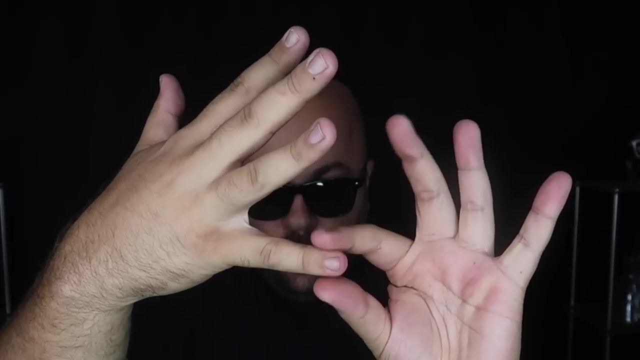 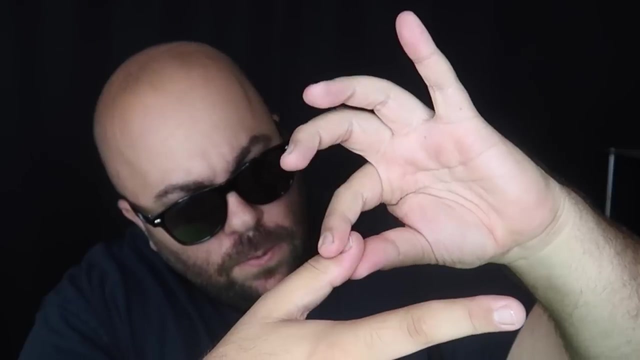 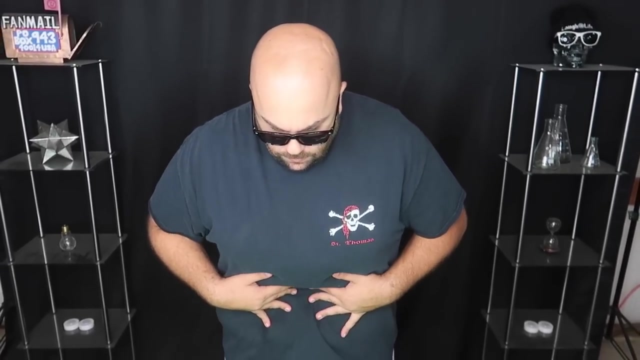 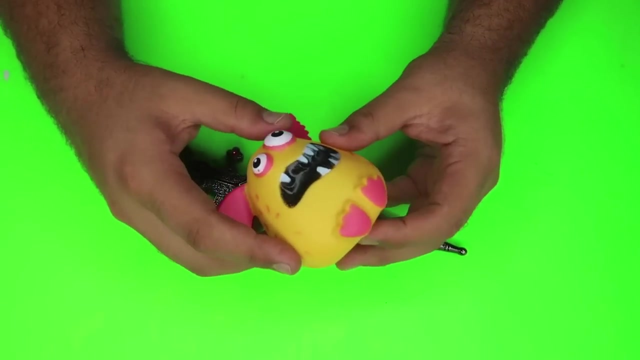 beautiful thing about this is you can then pull your hand out, show your hand completely clean. Here is the secret to the magic squeaky hand trick. You're going to need a pair of scissors and a dog toy- a squeaky dog toy. You can get these for like a dollar at Walmart or Dollar. 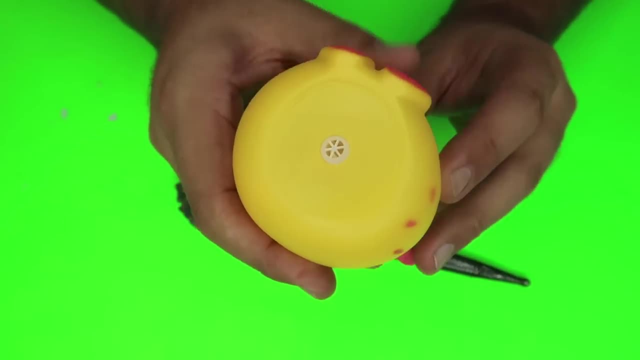 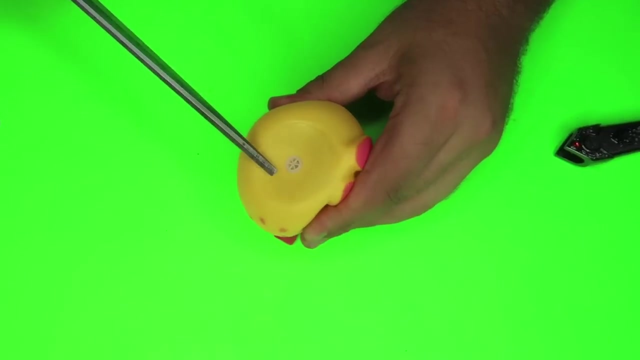 Tree Dollar General store And it has a squeaker built into the bottom of it. So when you squeeze it, air is forced through this little nozzle right here and it creates a squeak sound. So we're going to take our scissors and we're going to squeeze it, And we're going to squeeze it And we're going. 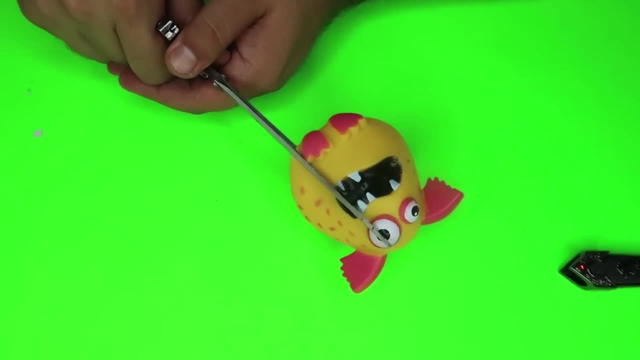 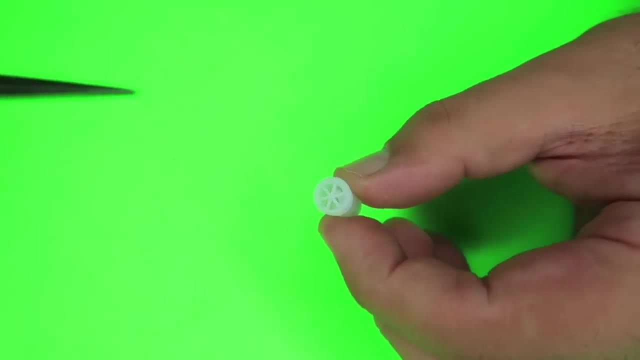 to remove the squeaker Carefully, cut the toy in half And once you get it opened up, you will see the little squeaker right there and you can just pop it out. All you need is this little plastic piece right here. Then all you do is pop this in your mouth and hold it between your teeth. You're. 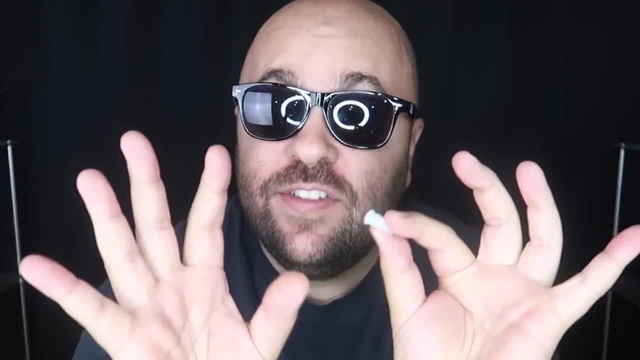 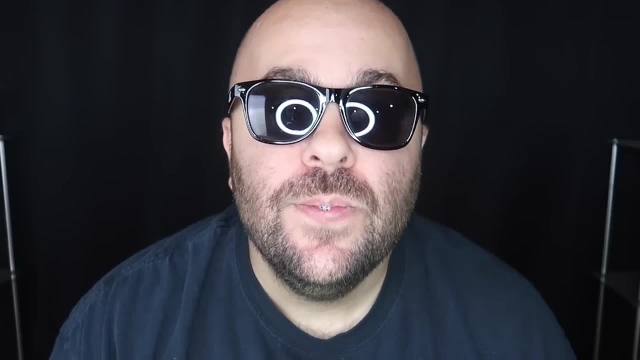 going to conceal it with your lips. Please be aware this is a choking hazard, so be extremely careful. You're going to put this in your mouth right here. As you breathe through it, the air passing through the little reed inside makes a squeak. 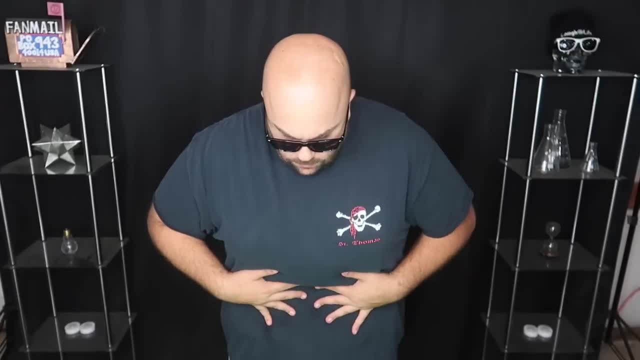 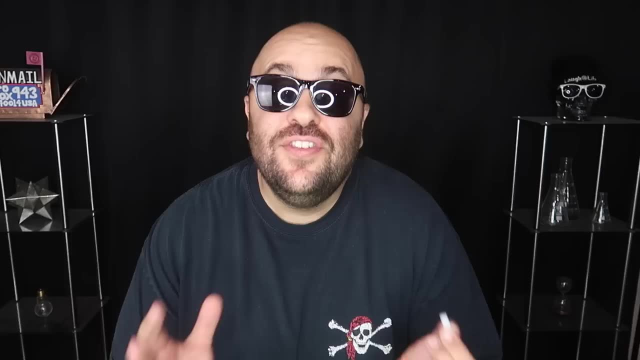 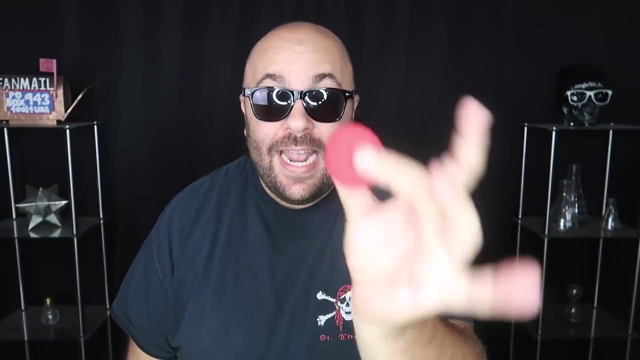 sound. So we can use this to make our hands squeak, our fingers squeak our stomach, really anything. You squeeze your ear, So just work on the timing of making your squeeze motion match the sound. You can do it with a sponge ball: make it squeak, then hand it to your audience and it doesn't. 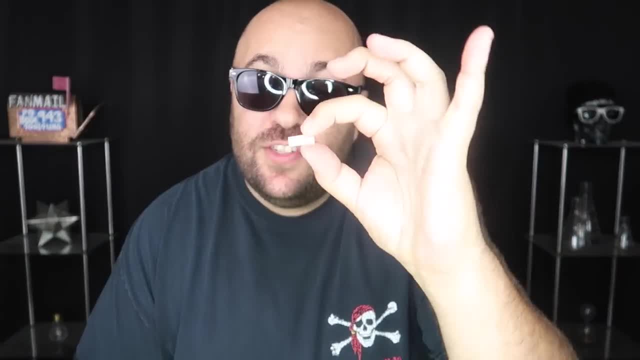 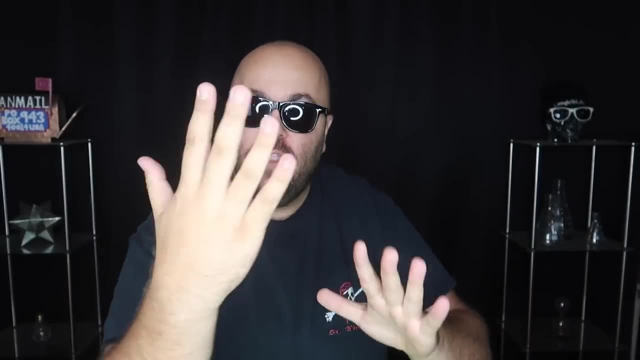 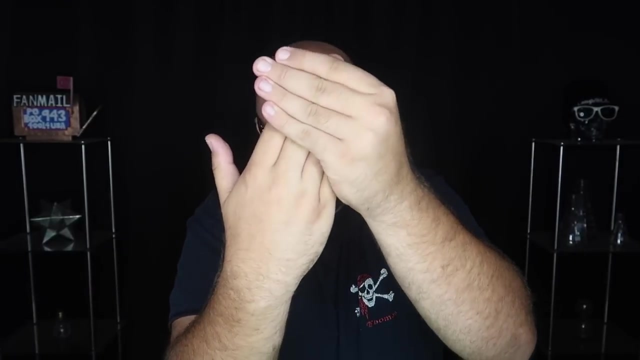 squeak when they do it. The possibilities are endless with this, So get yourself a squeaker toy and try it out today. An amazing hand trick that you can do anytime, anywhere. So check this out. Empty hands- I take my fingers like this Watch. I can actually just pull that finger off of my hand, just like. 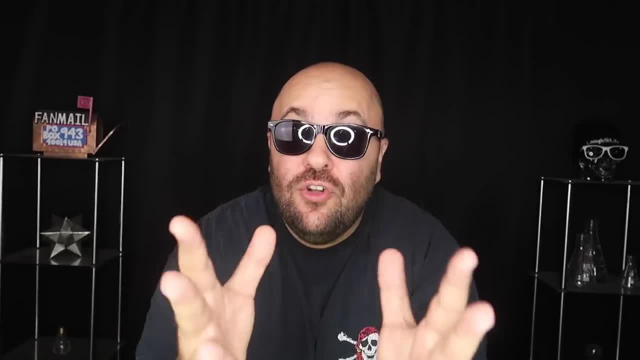 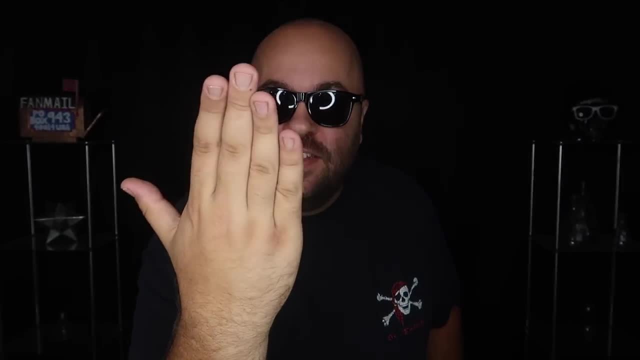 that, And now it's magically restored. This is a super easy trick, So it should be a really easy walkthrough for you guys. This is all about timing and speed, So you're going to practice this move When this hand comes down in front of the other hand. here's what they're not seeing: This finger. 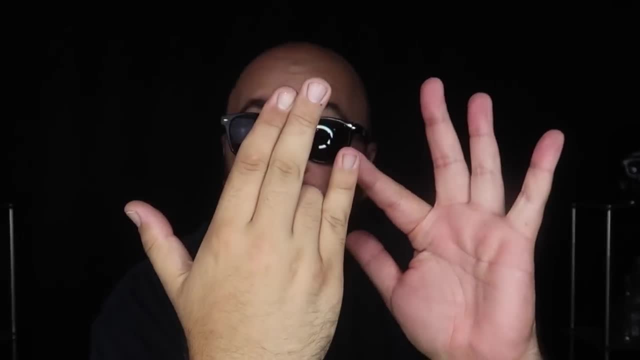 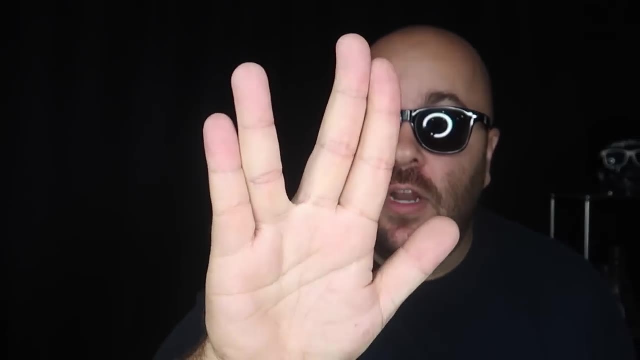 is going to fold down at the first knuckle right here, So it looks like your finger is just cut off right here. Now you're going to practice this move. As the hand spins towards the audience, that finger is going to come up and these fingers are going to split right in. 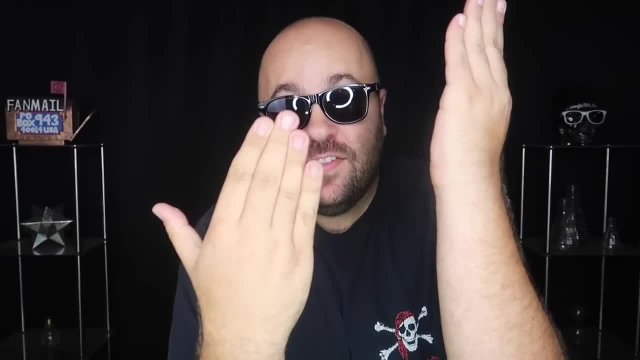 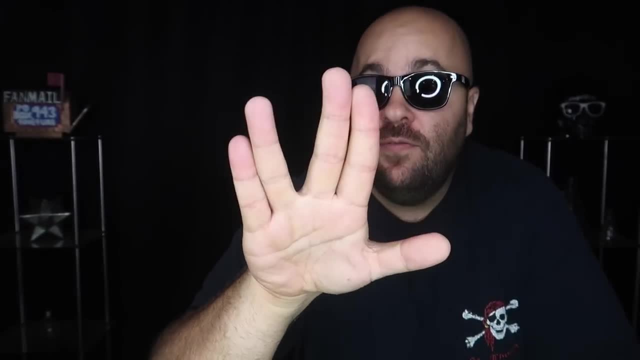 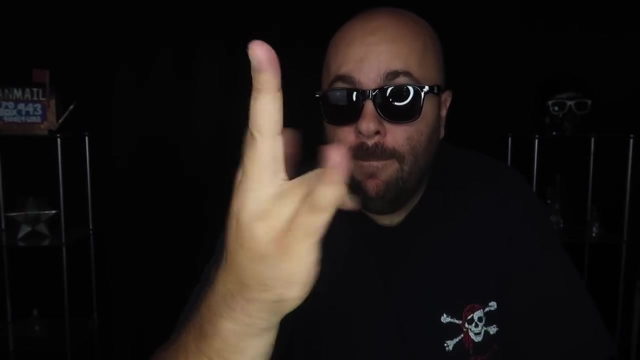 the middle, like you're doing the Vulcan sign: Live long and prosper. So practice your timing. As this hand comes in front, that finger folds down, And then the second part. the part you really need to practice is as the hand flips, the fingers split and then back: Boom, boom, boom, boom, boom boom. 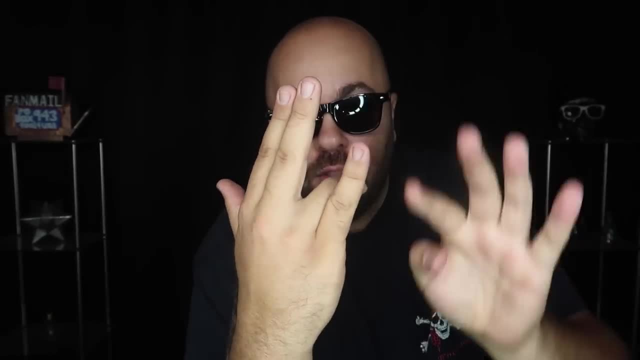 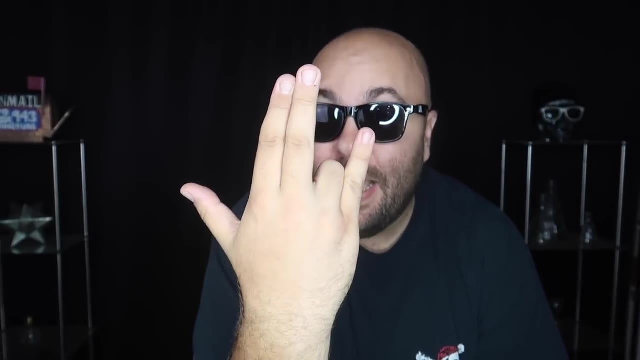 So what's really happening is you're creating this illusion of this gap here on the other side. You don't want to hold it too long, though, on this side, because then they'll realize that all four fingers are up. So just a quick flash on this side and then back to here, Just sells it in the 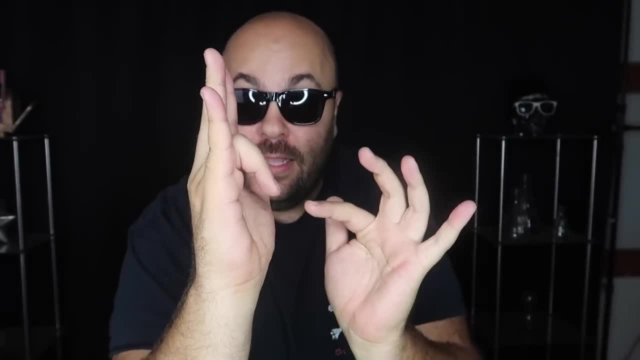 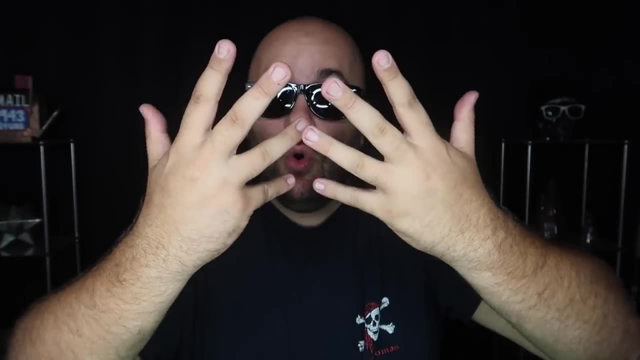 audience's mind that your finger really is missing and it's not just folded back like this And then it comes back over. You simply extend your finger up under the cover of the hand and boom, it's magically restored. A simple hand trick that you can do right now. Here's a really amazing and easy. 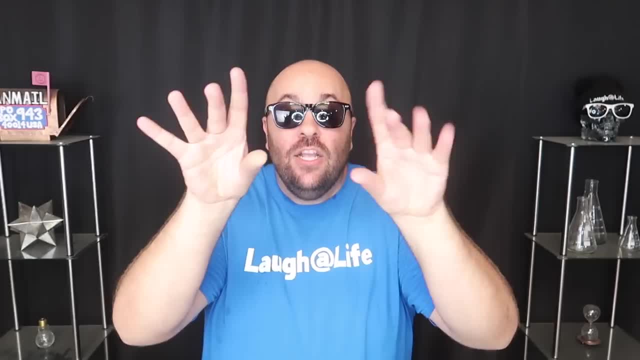 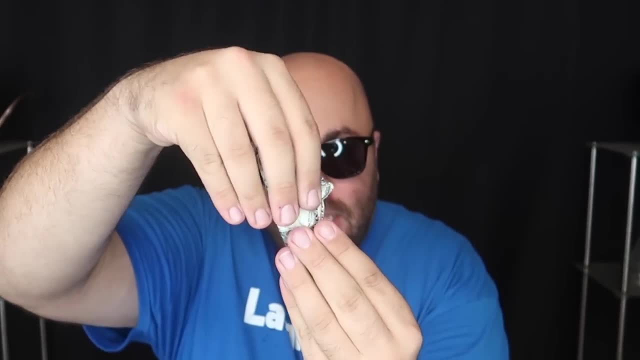 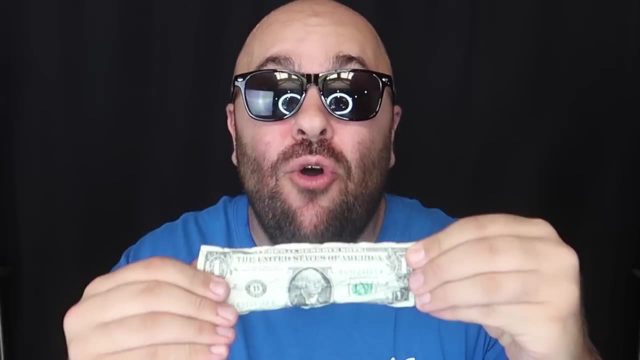 magic trick you can do with bare hands. Show your hands empty, front and back, just like this. Now look, if you could really do magic, wouldn't you make money? I know I would. I'll teach you exactly how to do this at home, coming up next. Here is the secret to. 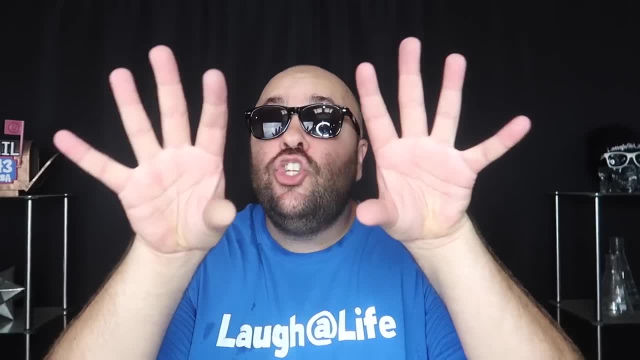 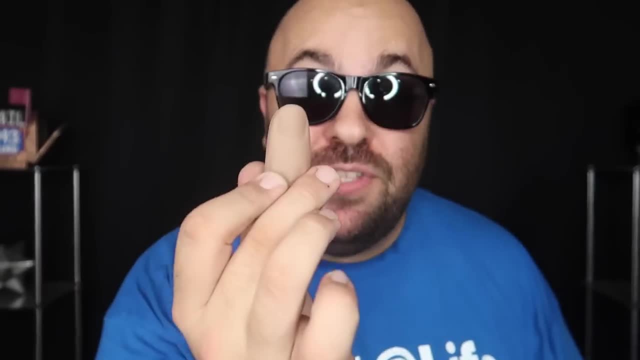 making a bill appear from your bare hand, When I showed you empty hands. that was a lie. There's actually a fake thumb right here. This is called a magic fake thumb tip. We have these available at evanairatvcom- That's our online magic shop. We have them available in adult sizes and kid 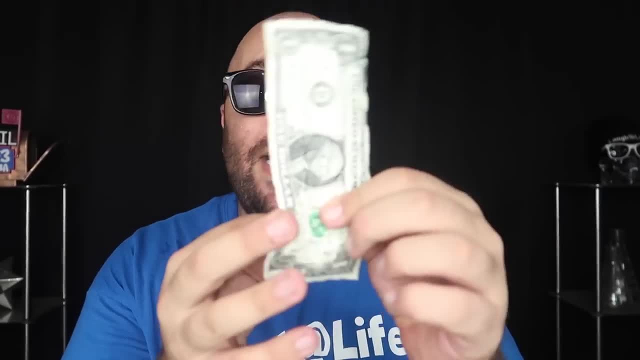 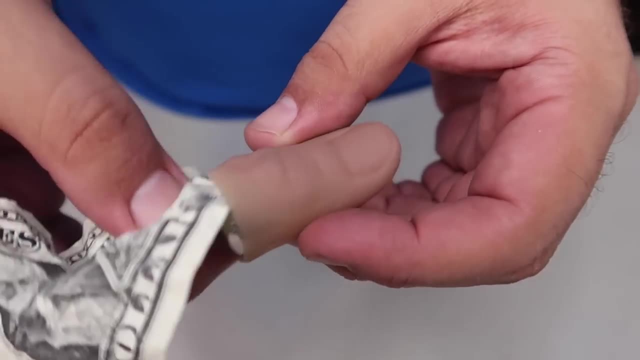 sizes. You can do thousands of different magic tricks with a thumb tip, But one of the easiest things to do is to make something appear. Stay tuned if you want to win a magic thumb tip. I'm giving five away at the end of the video to lucky comments. So take a dollar, stuff it inside the thumb then. 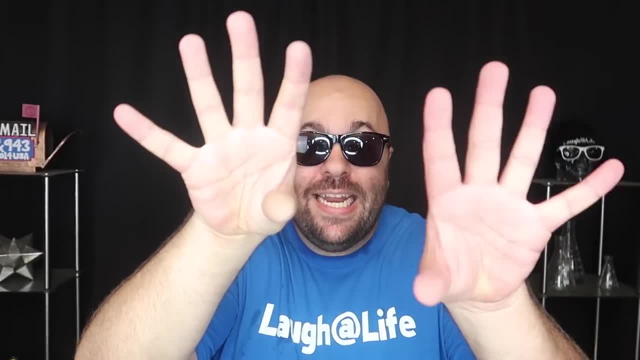 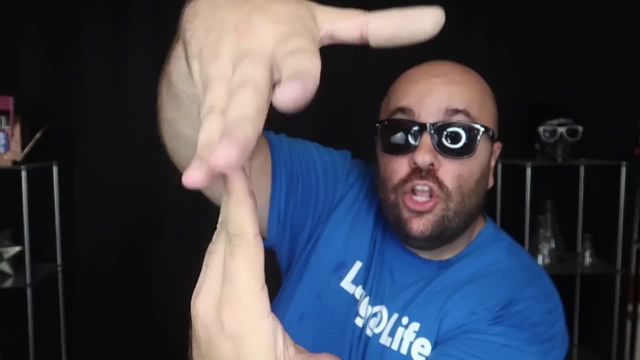 you're gonna put that thumb on just like this. Keep that thumb pointed at the audience, Don't show it like this. You're going to show your hands empty. You can show them front and back, and then you're going to come into this position, just like this. You're going to grab the thumb tip with your bottom. 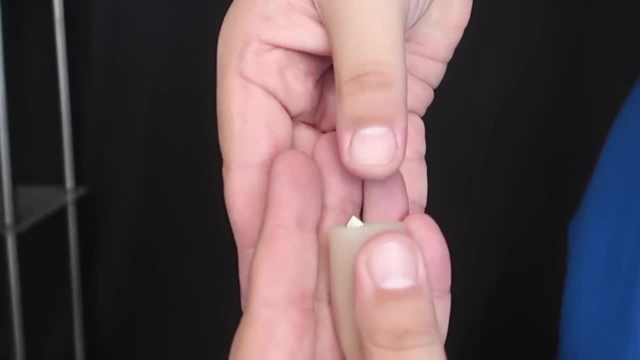 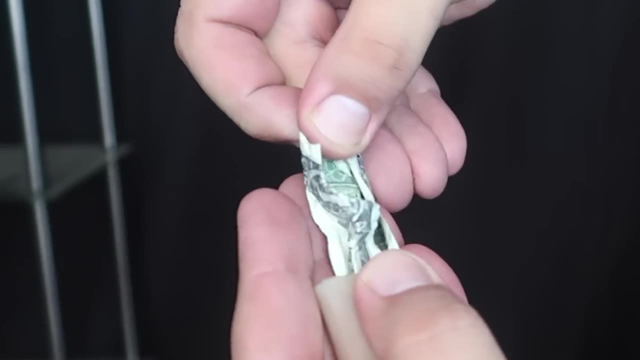 hand. Here's a backside cutaway view that the audience is not seeing. So the hand comes down like this, pulls the thumbtip off here, and then you're going to begin to slide that dollar out just like this in between the hands and kind of just let it uncrumple, just like that, and you're going to palm. 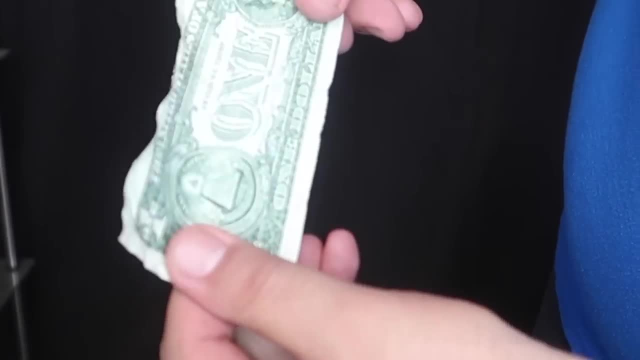 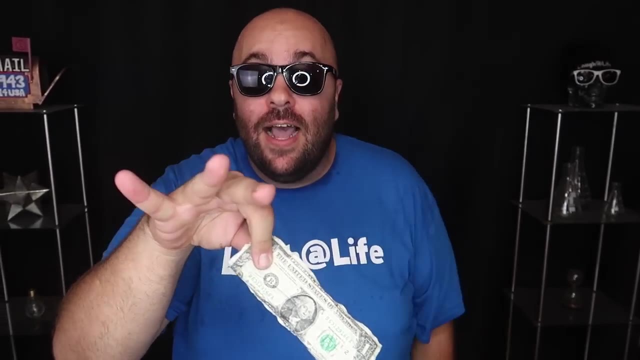 the thumbtip in the opposite hand, right here the entire time. then, when you hand this bill out to the audience for examination- and all of their focus is here- it's the perfect opportunity to drop this hand to the side, ditch the thumbtip into your pocket or you can simply slip it onto. 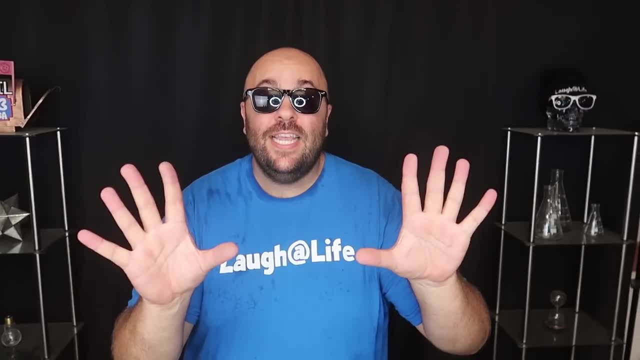 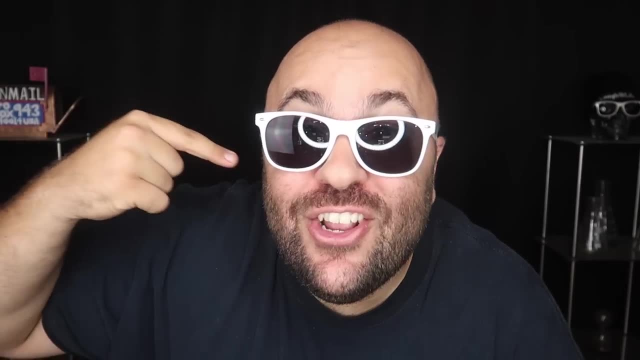 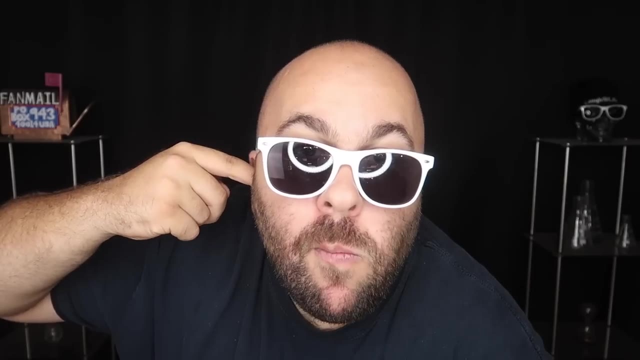 the thumb of the other hand. then you're free to show your hands completely empty and clean and take your round of applause. all right, it is bonus trick time. it's an extra magic trick for you. take your finger and put it in your ear, watch what happens. you can actually do it on the other side. 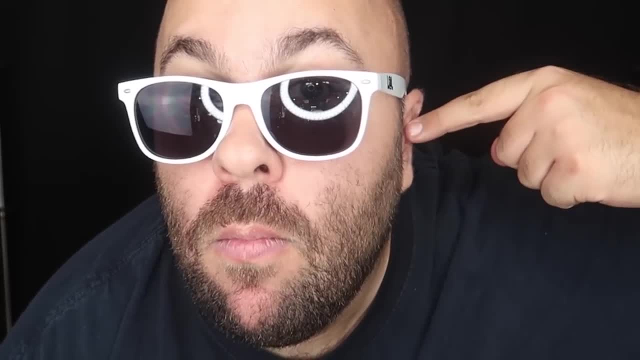 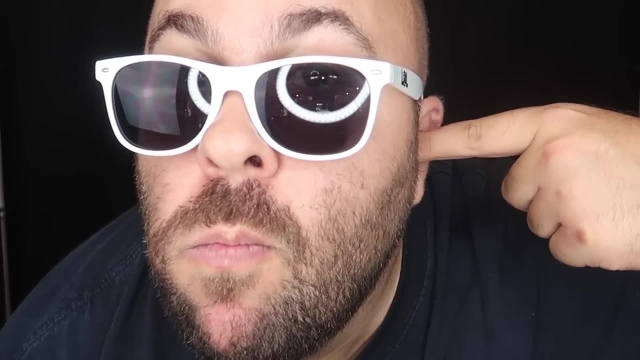 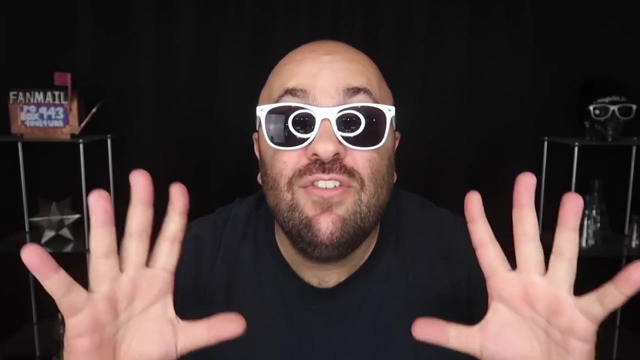 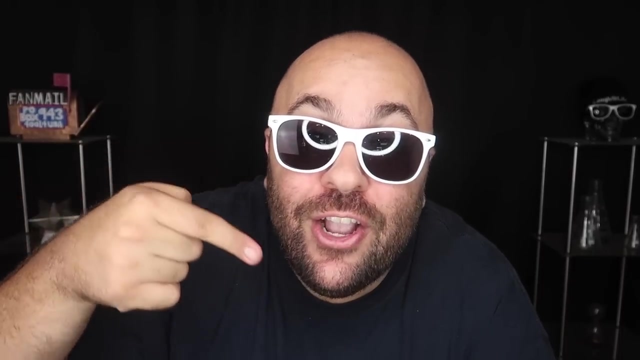 too. so the secret to this one is really simple. you're just using your tongue inside your mouth and pressing it into your cheek in time, with you pushing your finger into your ear. don't press too far, you don't want to hurt your ear. let's start out like this and kind of move it in like: 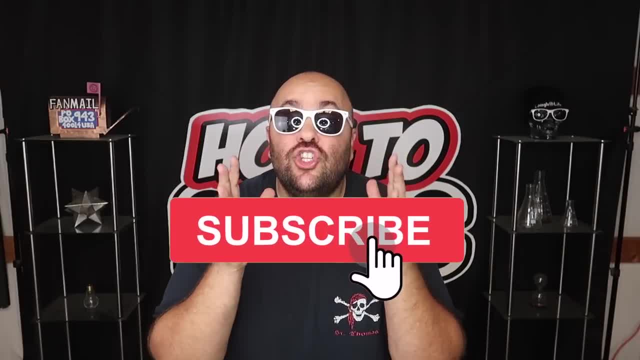 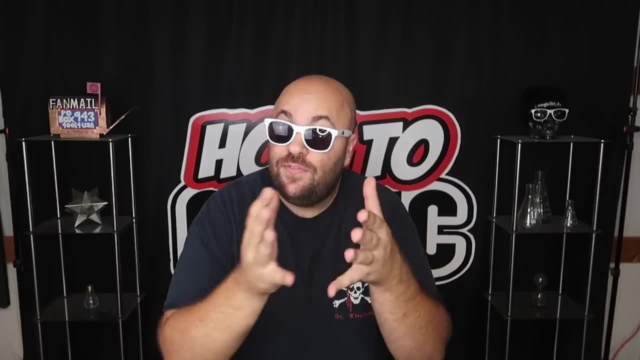 that, combined with sticking your tongue into your cheek. if you are new to the channel, please hit that subscribe button. almost 80 of the views on our channel come from people who are not subscribed to the channel, so if this is your first time watching the video or if you're new to the 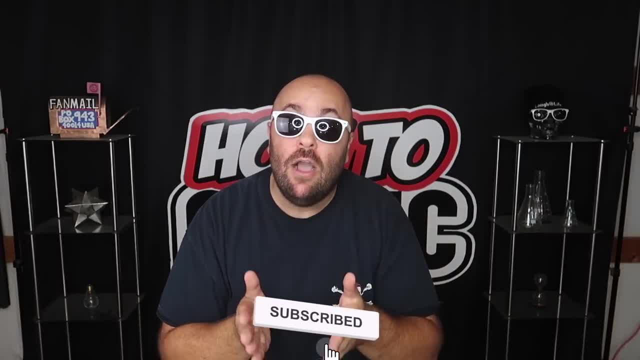 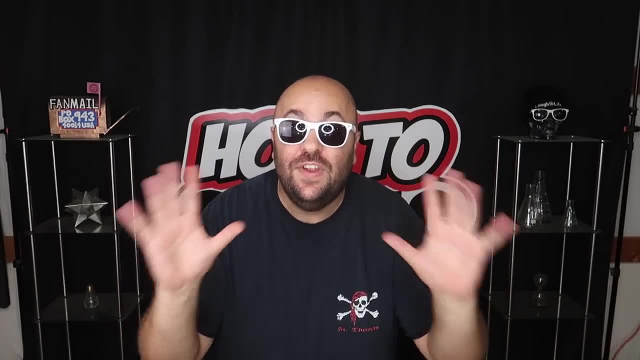 channel. if you're watching and you haven't subscribed to the channel, please subscribe now. you can get notifications every single time we post a new video, and it is giveaway time. i am giving away all the magic props from this video, that is, five magic thumb tips to lucky comments. 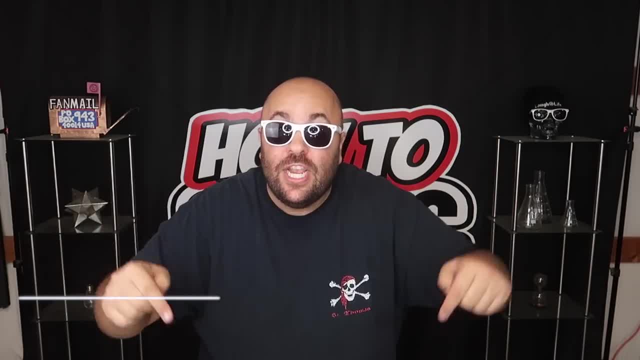 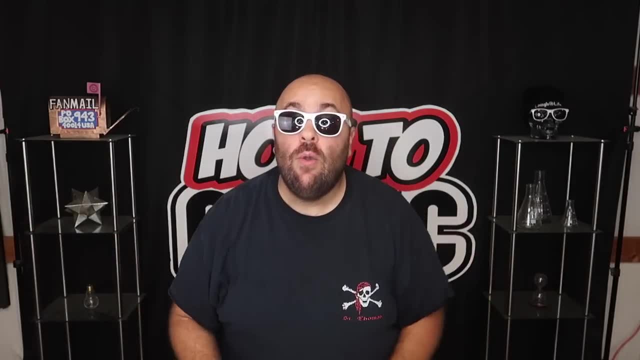 in the comment section down below. all you have to do to win is be subscribed to the channel and leave a comment down in the comment section. i'll be going through the comments and choosing random comments and mailing out the magic to you. time to announce the giveaway winners from the last how. 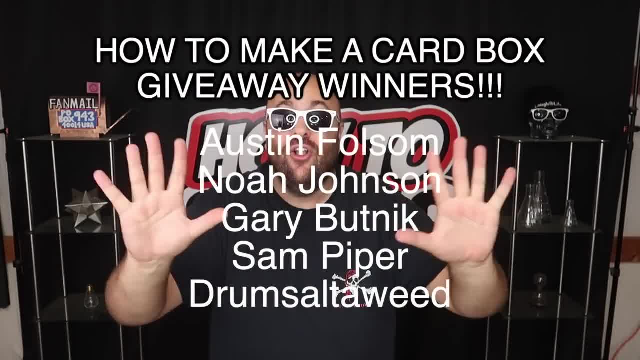 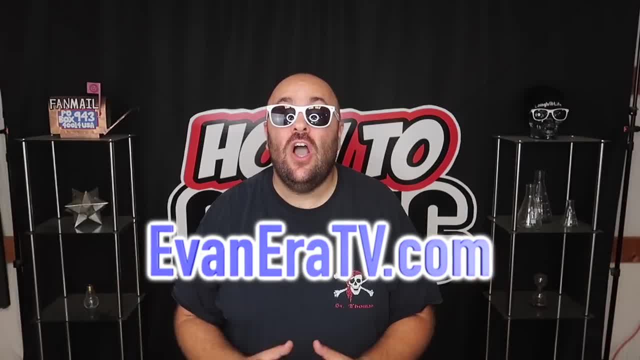 to magic video. the winners are appearing on the screen right here. congratulations to our winners. check the description of the video for instructions on how to claim your prize. be sure to check out evanera tvcom. that is our online magic shop. you can get magic thumb tips. 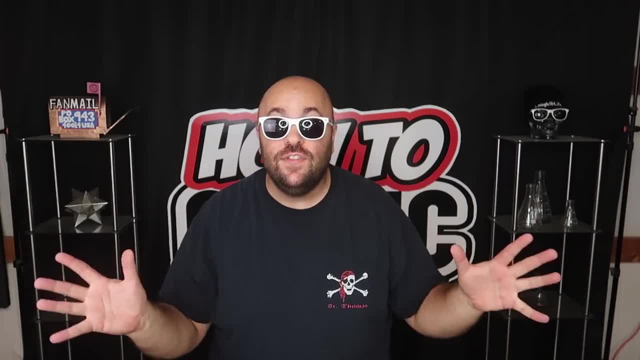 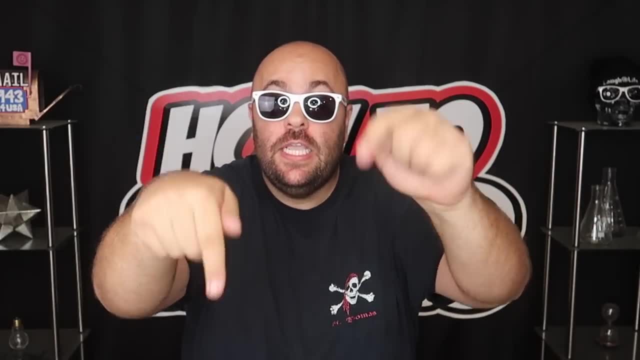 and a ton of other really cool magic tricks, and we ship them all over the world. so no matter where you're watching from, you can get a big box of magic delivered to your door. the link for that is in the description at evanera tvcom. if you missed the last episode of how to magic catch. 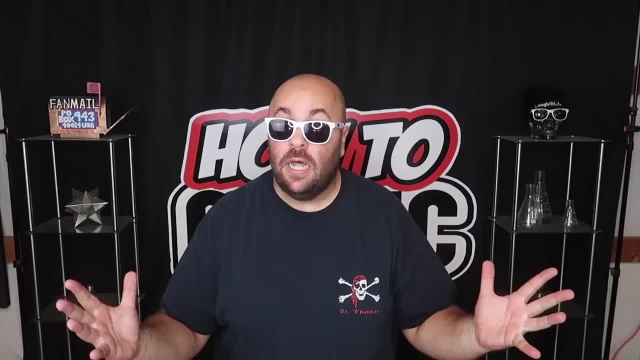 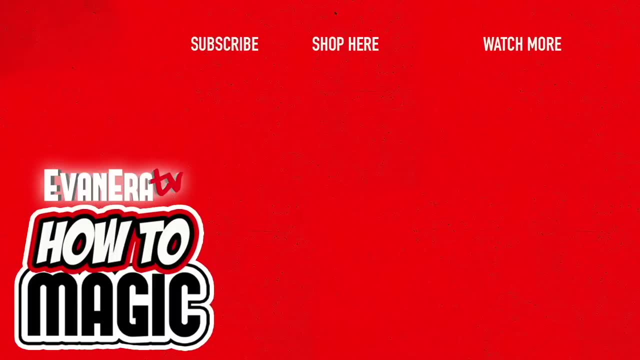 up by watching it right up here. and until next time, remember that anything is possible as long as you stay positive, work hard and laugh at life. love you guys. bye.